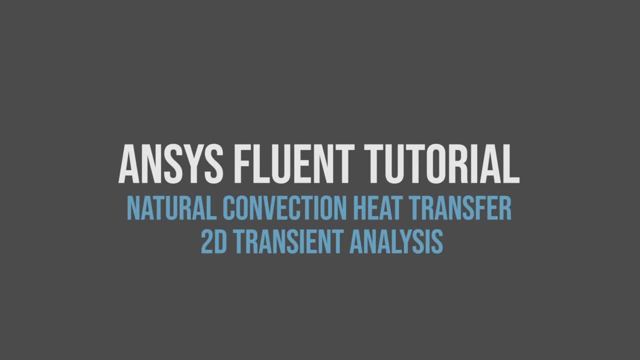 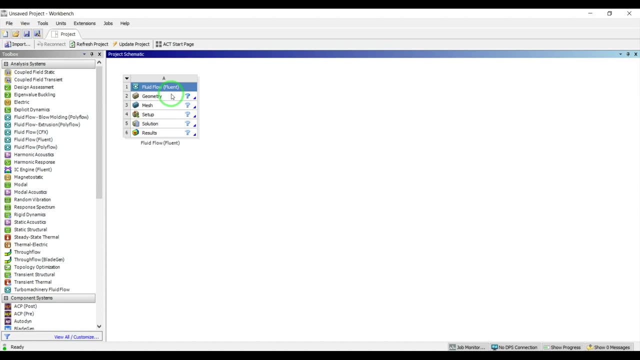 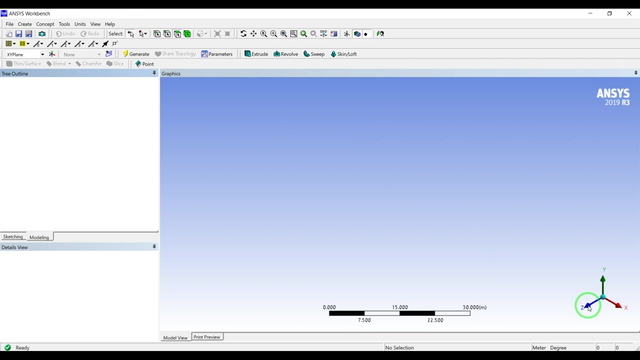 Hello everyone, in this video I'm going to show you how to do the natural convection simulation using ANSYS Fluent. So I have created a block with the Fluent flow here and I will open the design modeler and to create our geometry. So first I will go to the M units and change my units to 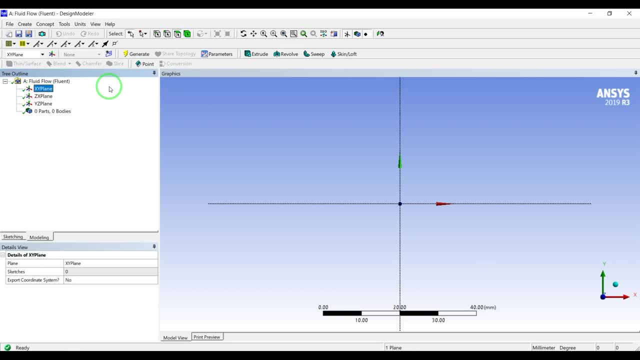 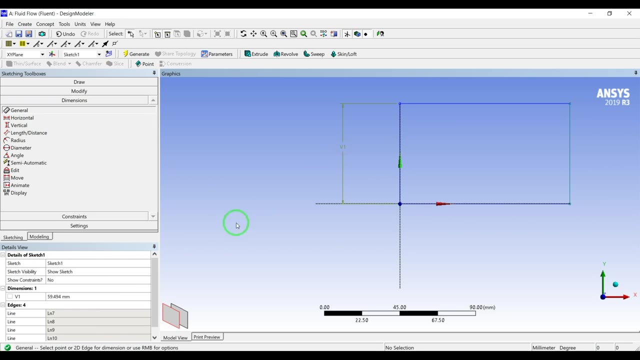 millimeters and go to XY plane to create a new sketch. So I will create a rectangular. so let's do the dimensions as 80 millimeters and under 20 millimeters. So here I will draw some rectangles. Let's do this method. 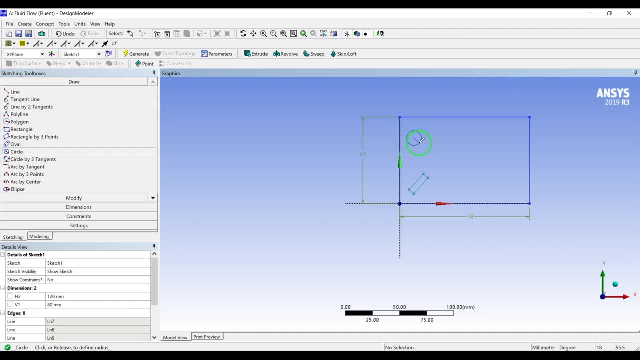 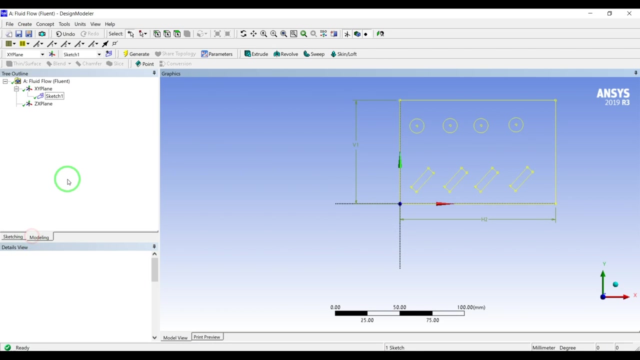 And the circle. Okay, then I will go to modify. First I will select the circle and four sides of sides of these rectangles by holding the ctrl key, Then click on the copy and I will make four copies of these circles and rectangles. So then press escape to finalize the copy, I will go to modeling and since I'm 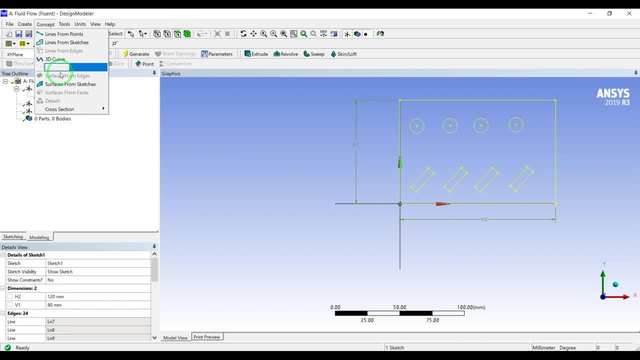 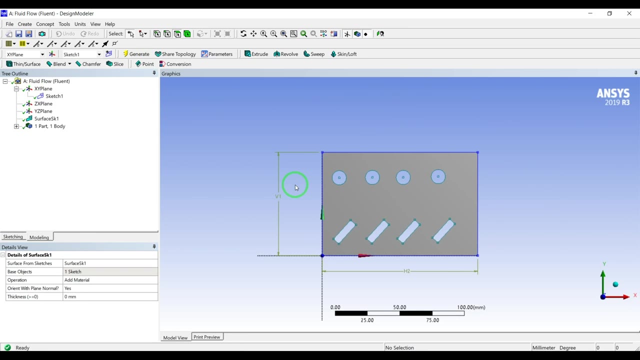 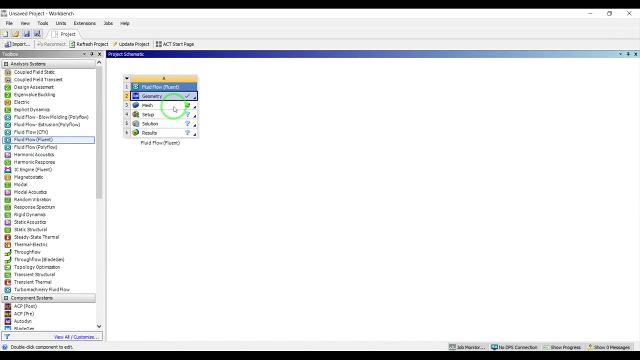 doing 2d simulations. to do the faster simulation here I will do the concept surface from sketch Okay. this sketch is selected and I will press generate. So I have my geometry. I will go to the meshing So I'm going to create one of these. 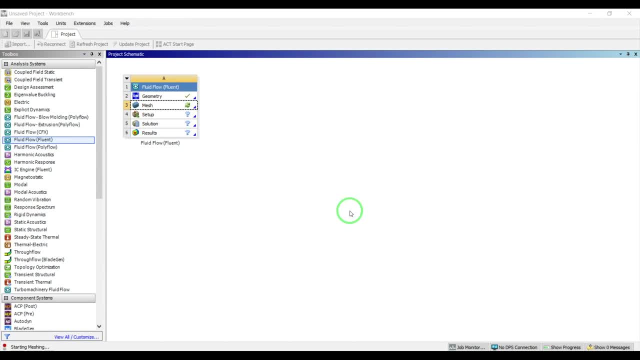 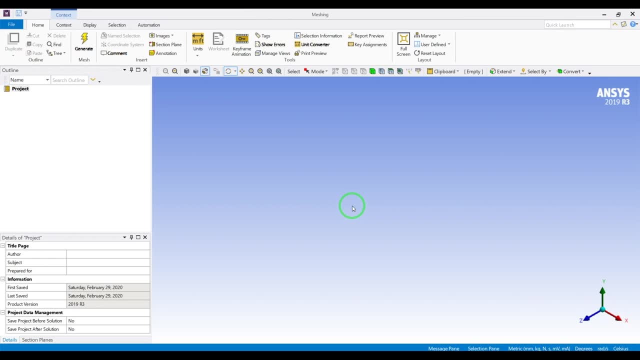 So I have my geometry. I will go to the meshing. Here I will try to create a very quick mesh, but I'll just cut this out here. and here I will try to create a very quick mesh, but I will just cut this out here. and 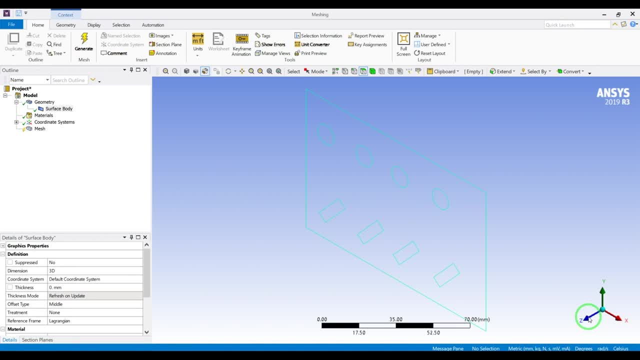 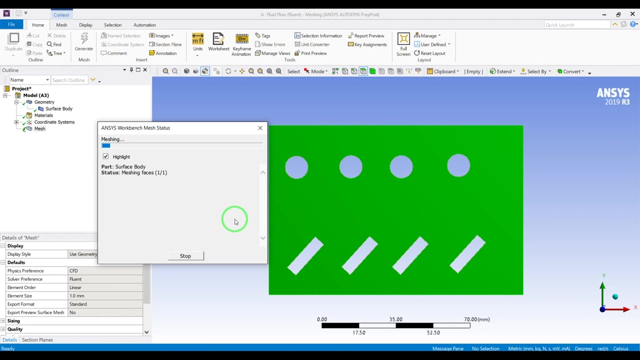 and I will also explain, if you want to go for more details, what you can do. so let's do the size of the elements as set as one millimeter. so let's generate the mesh and see how it looks like, always using some coarser mesh, and see the general mesh. it's better to. maybe we will better understand. 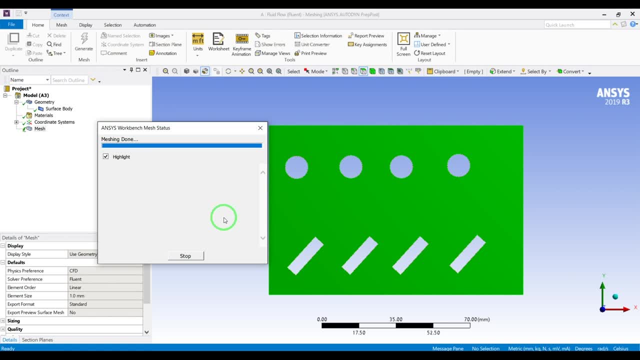 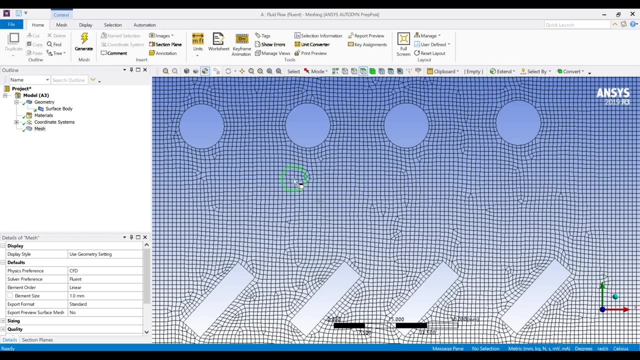 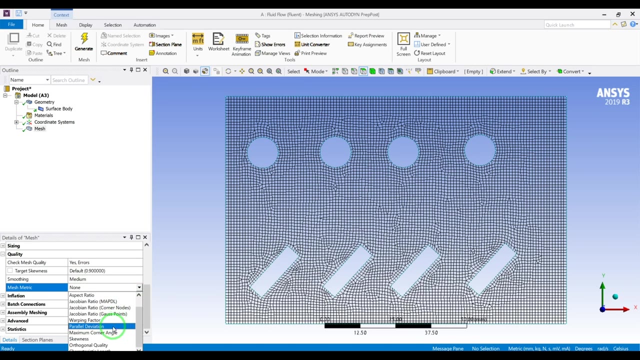 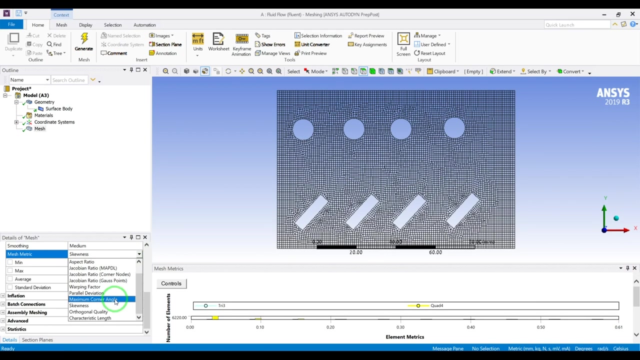 and the complexity of the geometry and generate our mesh, refine the mesh based on that one. so it looks like a pretty decent mesh. so let's check the mesh metrics from the quality. so let's check the skewness and the maximum is 0.6, which is good. lower than 0.9 it's okay, and orthogonal quality: the minimum. 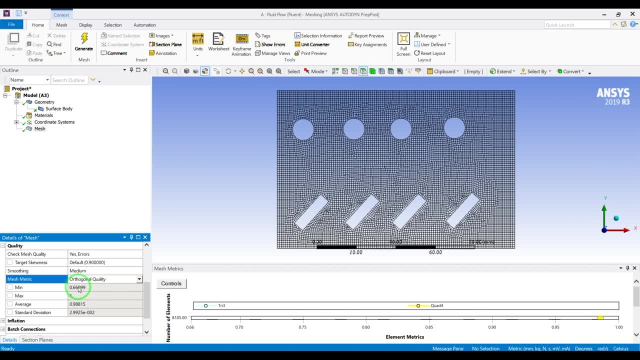 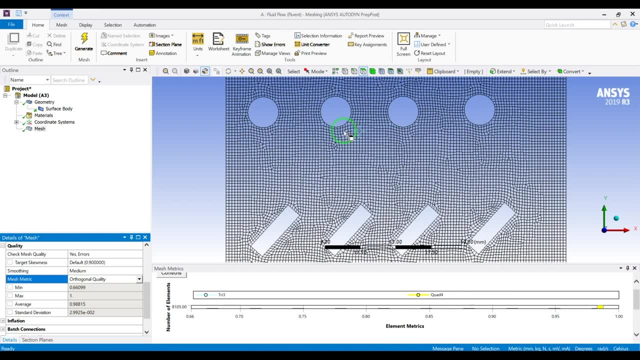 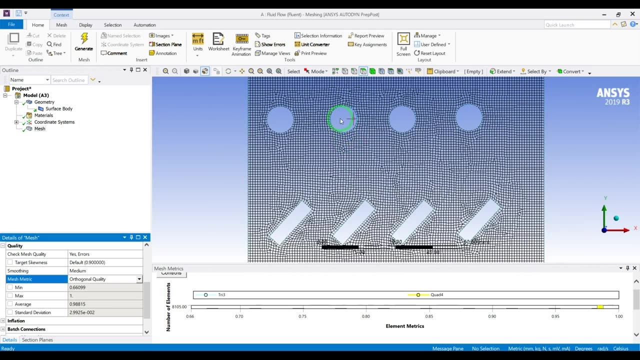 is 0.66, which is more than 20 or 15, will be acceptable for most of the simulations and also if you want to um, for example, study flow around the um wall or specific shape, it's better to have some inflations around that shape. you can right click here- insert inflation. 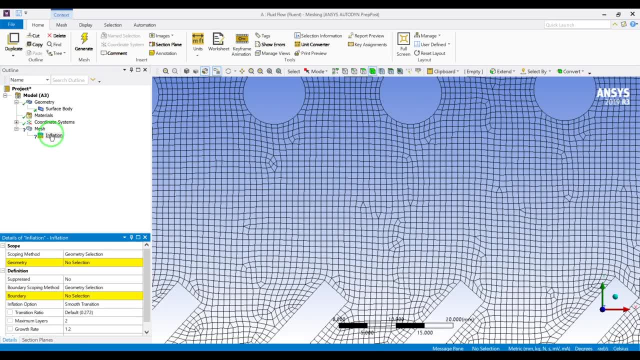 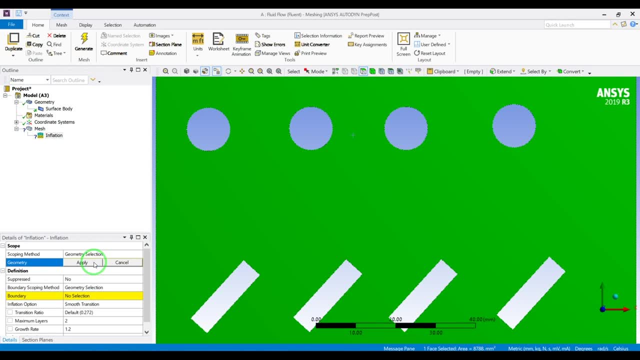 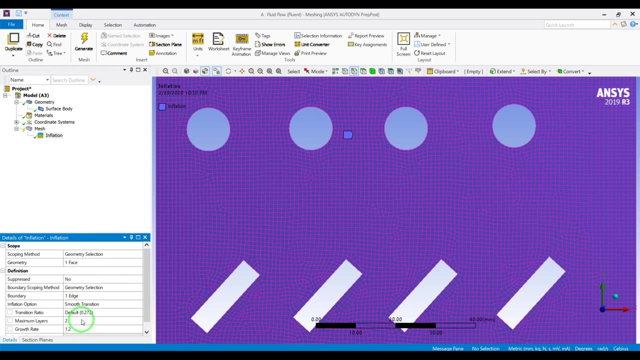 select that. um, I will create an inflation to just demonstrate, but I will delete that one rate later. the geometry will be our surface, which we are doing 2D, and the boundary will be: let's click this circle and apply like five layers of inflation, so let's generate the mesh. 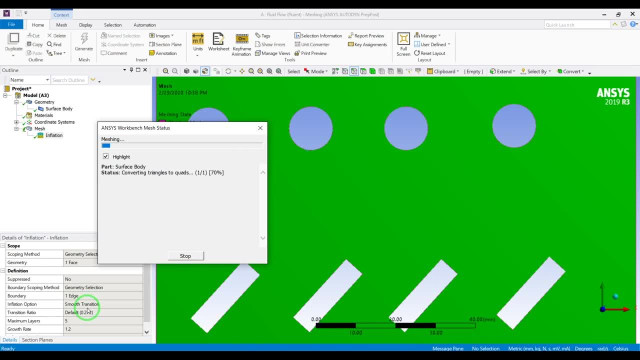 and the type of the transition is smooth transition. so you can define the height of first layer or um pace of maximum layer, based on your y plus or and based on your calculations. so this is more detail and based on each turbulence model you are using, based on your physics and those kind of stuff. 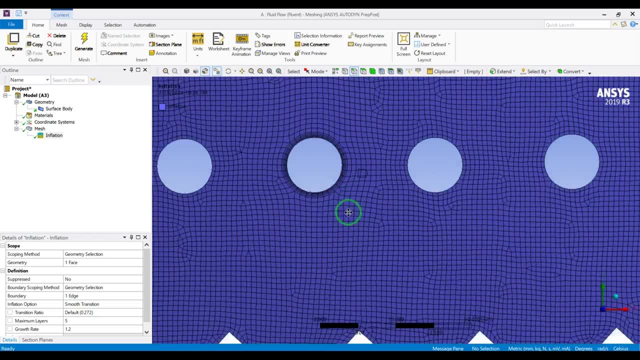 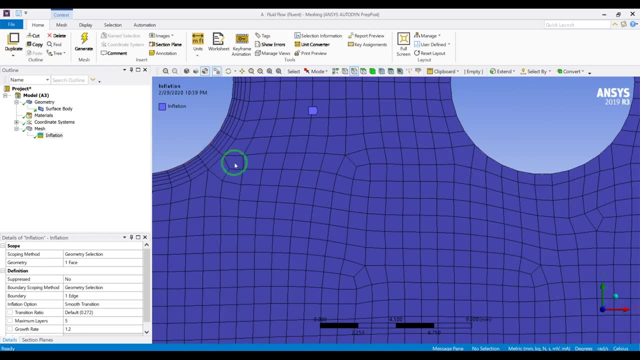 okay, our mission is done, as you can see, and for the other circles we didn't have any inflations, but for this one we have inflation, so we have finer measure on that boundary, so we will not need this one for our simulations. I will just delete that one rate, so you have to identify the unaffiliatedцию and replace it, so we need that one. 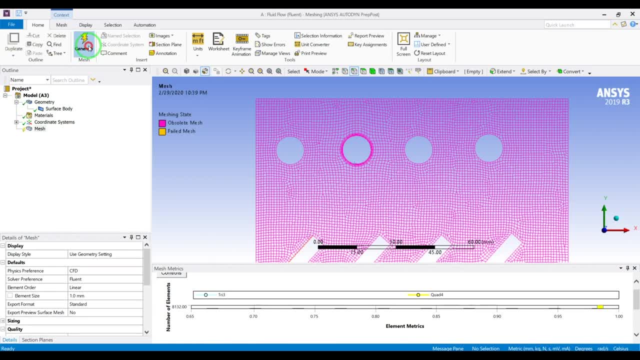 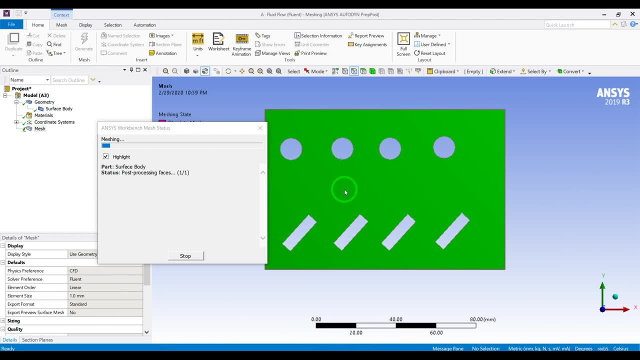 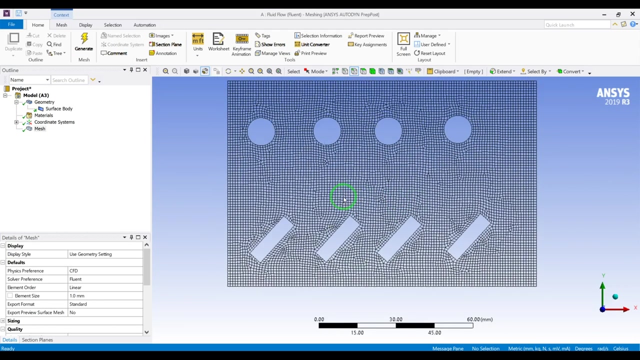 I will just delete this simulation and generate mesh again. You can based on the physics, as I mentioned before, based on what's your goal from the simulations. you need to have finer mesh around specific objects or if you have like higher gradient somewhere, you need to study that part more in detail. so you need to have a. 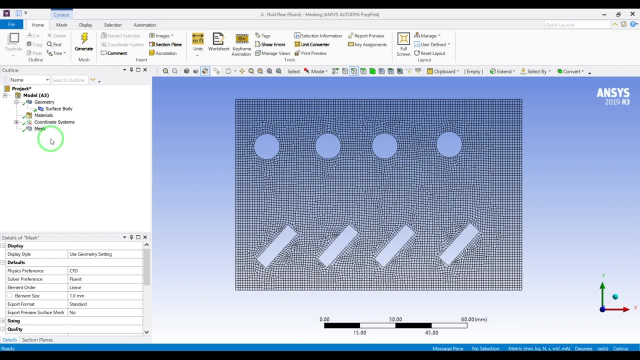 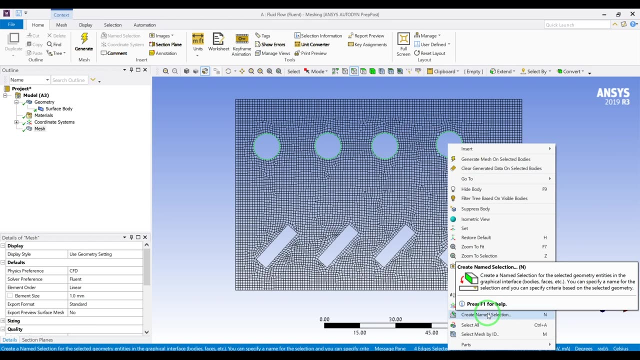 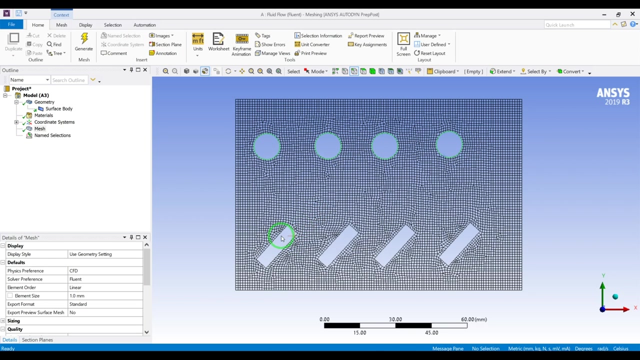 finer mesh and also based on the computational power you have. So now we will define, hold the control, define these, select these circles, then right click, create name selection circles and for the name selections, the creating name selections. 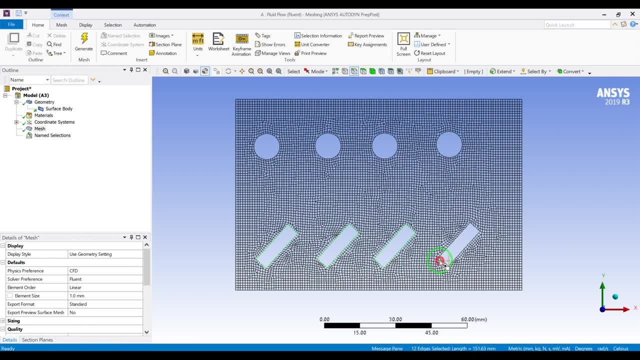 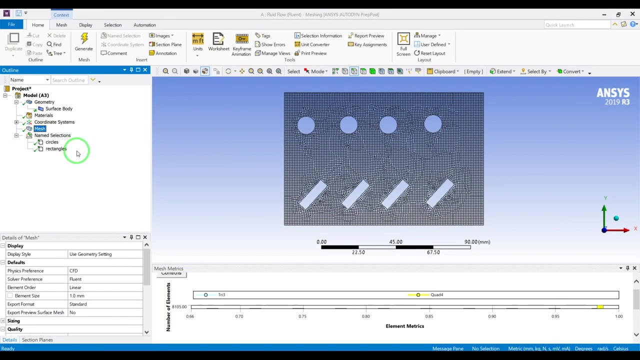 the shortcut is N, the letter N on your keyboard. so I hold control and selected these 16 edges as you can see here. then I will press N rectangles. okay, So we have our circles, We have our name selections here and here. so, and I right click update the mesh. so 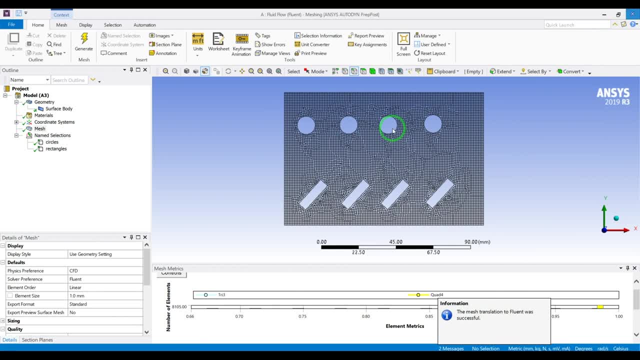 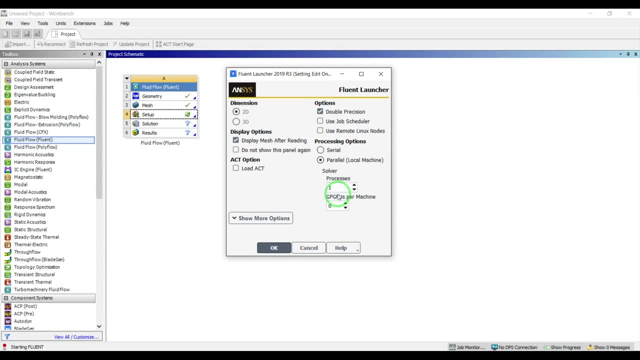 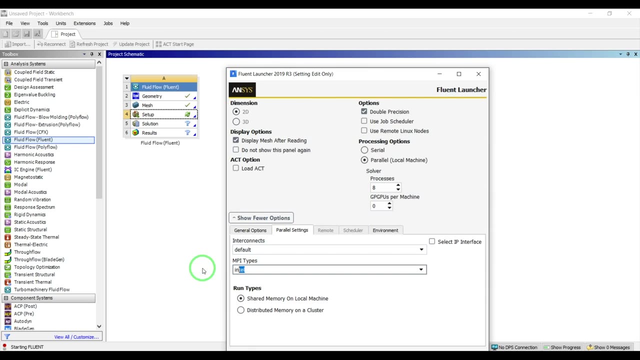 it will send the mesh to Fluent, So I will close this one. let's open Fluent and do our simulations. So I will use parallel mode 8 CPUs. I have an Intel CPU and also installed the Intel MPI, so that will make my parallel simulations faster. 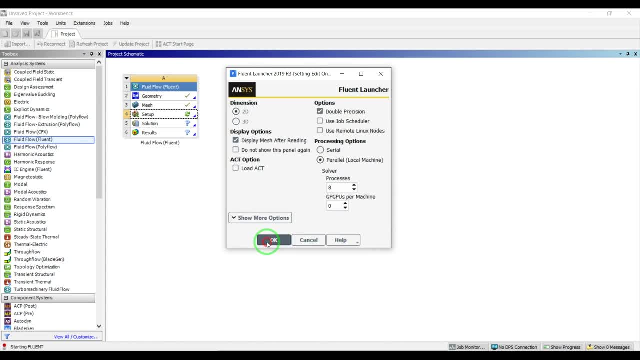 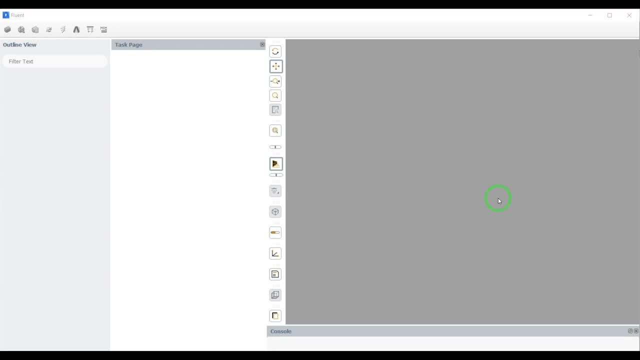 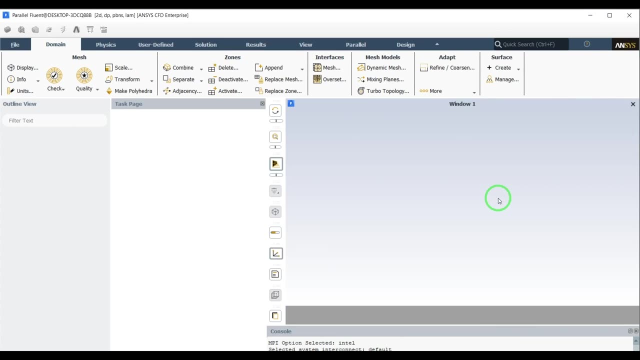 You can leave this one as default, So it's not that important. but if you have, if you are sure that you have installed the Intel MPI during your ANSYS simulations and you have- it's better to select Intel, because I, or if you have IBM MPI, it's better to select IBM. 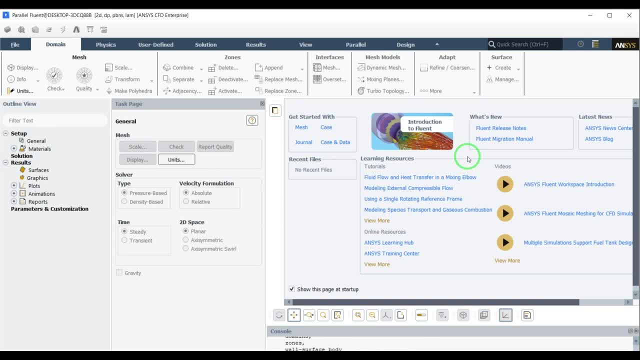 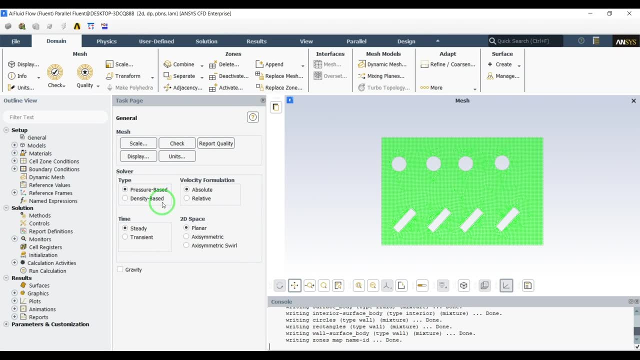 I have seen that it's making some difference in the simulation speed. Okay, We have our mesh here, So let's select transient simulations And, as you know, for natural convection is occurred by density gradient and, based on the gravity, we will have some buoyancy forces. 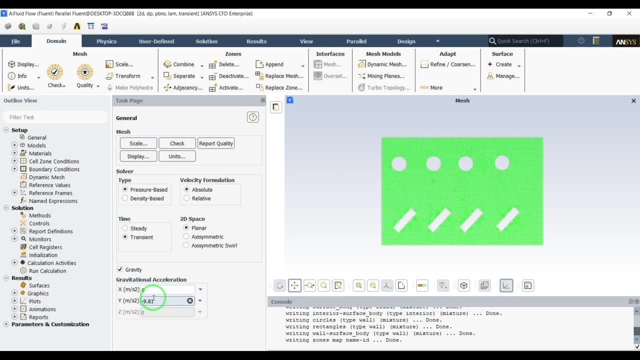 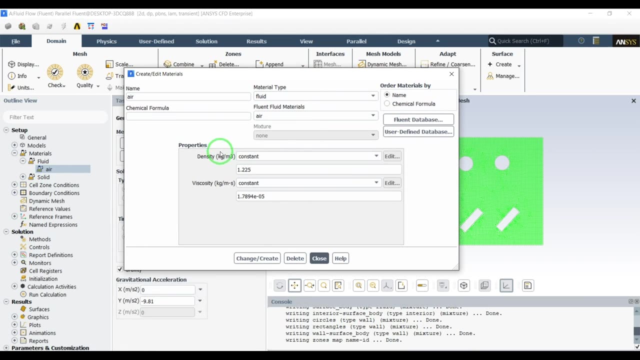 So having gravity defined in our simulations is in our simulation, is essential for the natural convection. So the other essential thing That is defining a material that it's density is changing by temperature, So as a default, the air, for example is, has a constant temperature. 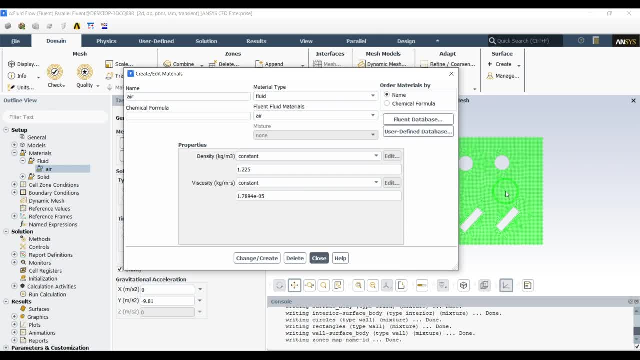 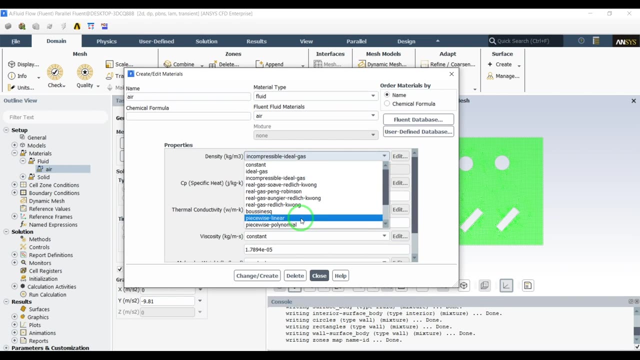 So if you do the simulation, you will not see any natural convection. The only thing you will see is the conduction. So it's better to change it for incompressible ideal gas. Or if you have another material. if you have a table, you can use a piecewise linear and 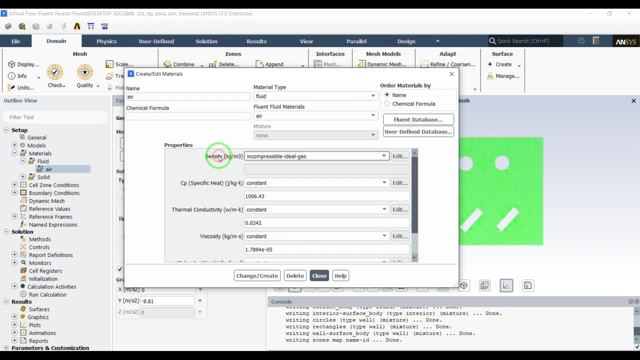 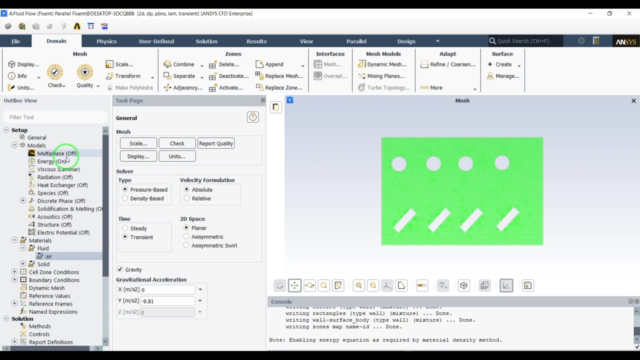 input your table here: the temp and the density versus temperature. Okay, Let's do create change. and it automatically enabled energy equation because we did the ideal gas, So I will leave it as is. For the viscous model, I will keep the laminar because I want to do the faster simulation. 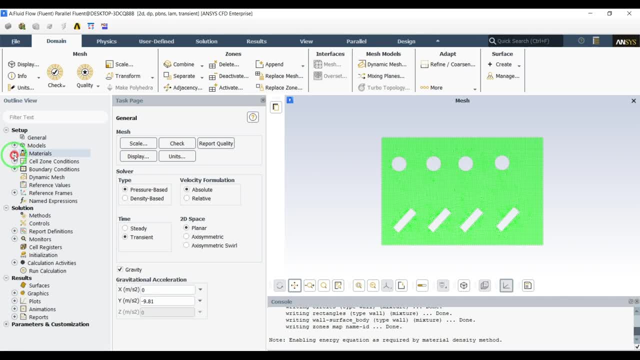 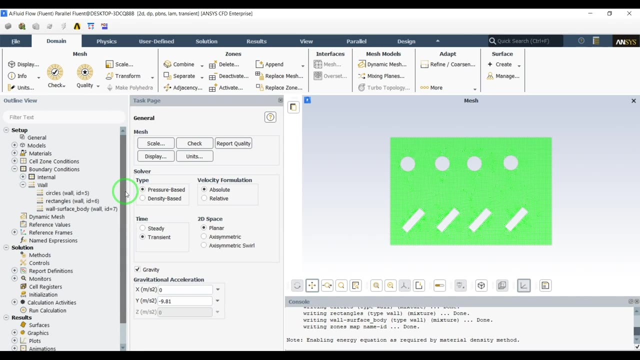 but based on the Okay- Okay For the physics you are simulating- you can calculate the Grashof number, which is like a Reynolds number for D- natural connection, And based on that you can identify the the nature of your simulations. 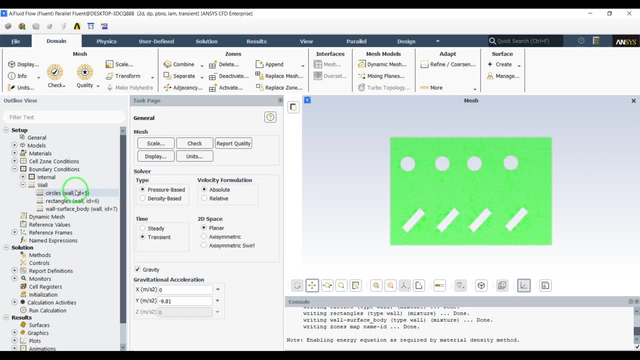 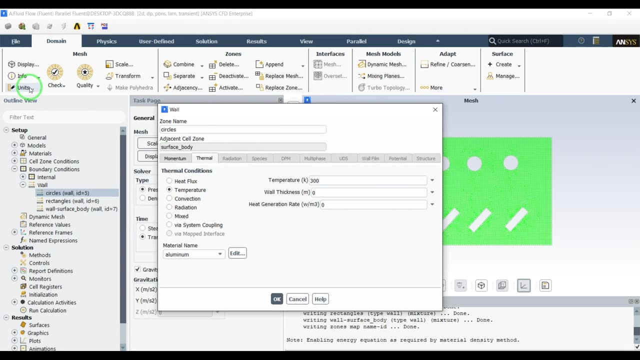 And based on that, you can select your turbos model model or keep it as it, as a laminar. Okay, Now let's define the temperature of the circles Simply as a temperature boundary condition. so I will change the temperature units here: temperature Celsius- okay, let's define them 20 as the 20 Celsius. all of the 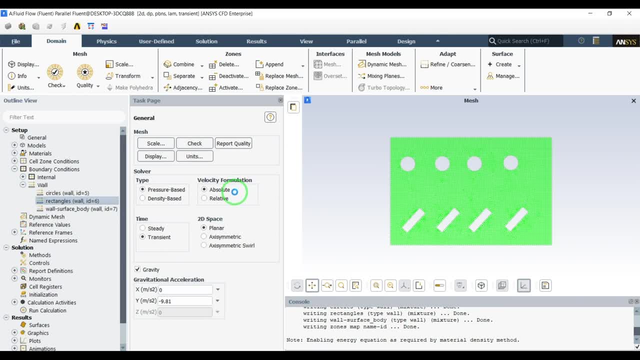 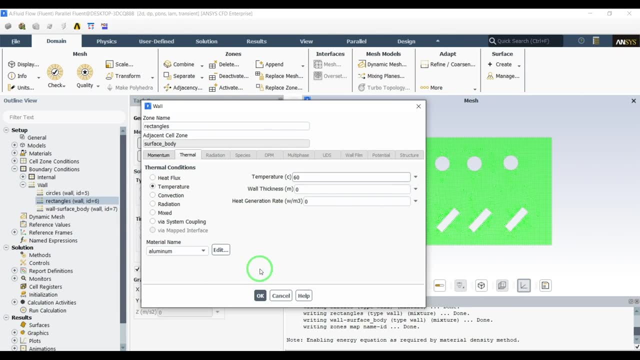 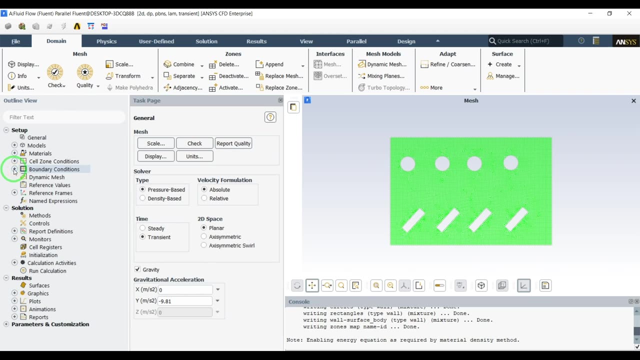 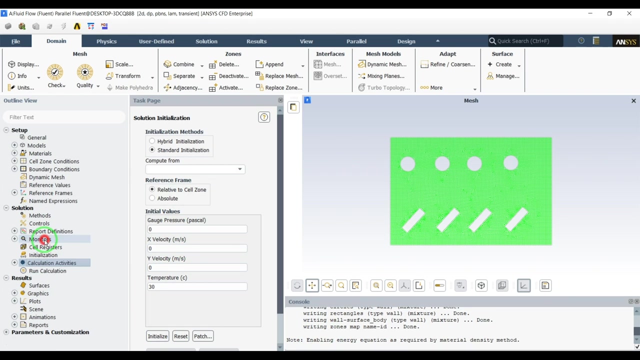 circles and all of the rectangles. let's define them as boundary condition of the 60 Celsius, so they'll have hot rectangles and cold circles here. so let's go to initialization. I will initialize a system at 30 Celsius, click initialize. so first let's go to calculation activities and save our 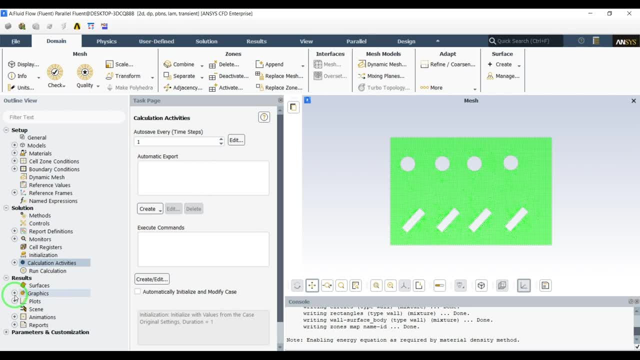 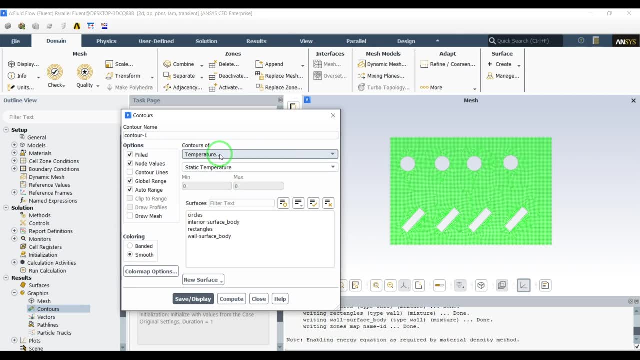 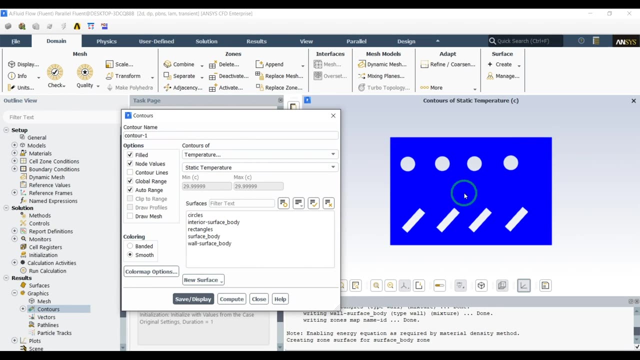 data every one time. step also. I'll save our data every one time. step also. I'll save our data every one time. step also. I'll want to see the temperature counters. so for 2d simulations, after selecting which counters you want to do, it's better not to select anything. so in this case you will have this, or if you. 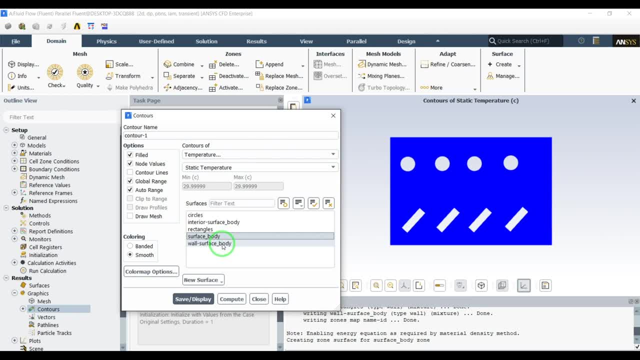 if you select, for example, um, let's see surface body, you will see the mesh in in your counter because it was common in all of the previous um fluent versions. so it's better not to select anything, you just press display so you will have the counter everywhere. also, i want. 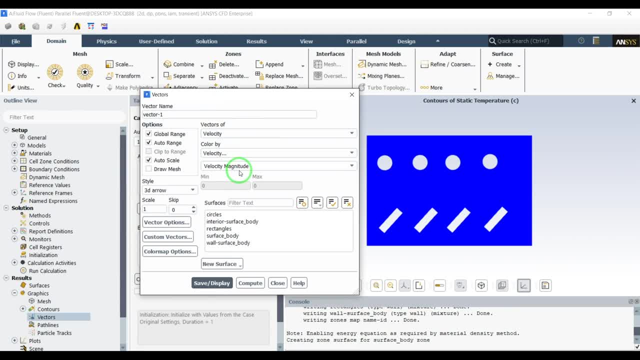 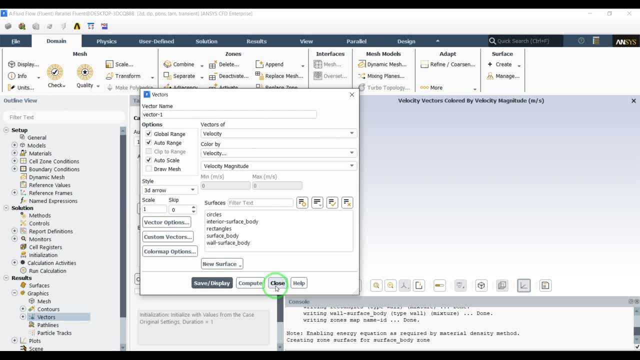 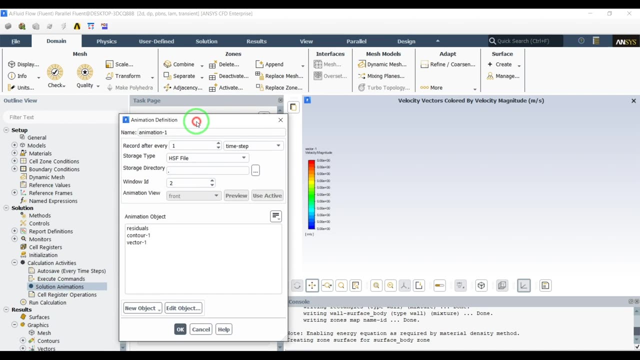 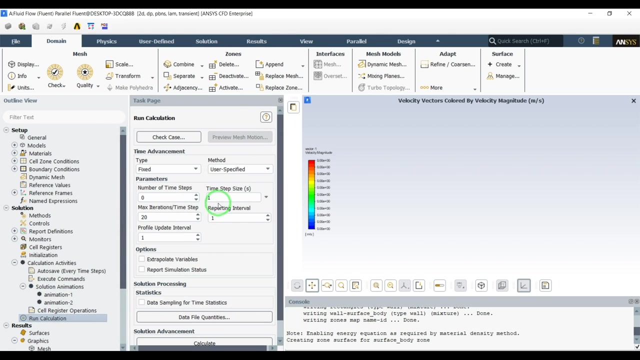 to see lost vectors. so let's keep this one as is and select, save and let's close this one. and from the calculation activities i want to see the animations of these counters, and the first one, this one and another second animation as the velocity vectors. then i will go to the calculations. i want to have a 0.1 seconds as the time step size and let's do a. 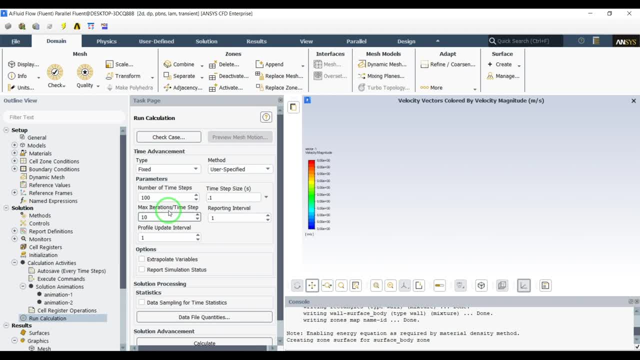 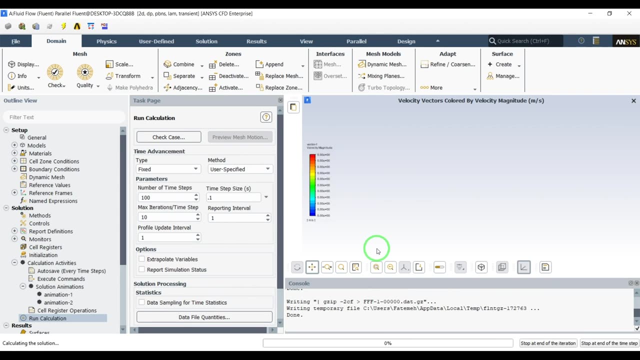 10 seconds, simulations and iterations, every um number of iterations every time, and every time steps 10. so let's do the calculations and, as you can see, for every time step it will create the velocity vectors, so that's um temperature gradient, temperature counter and animations, and also it's saving the data for. 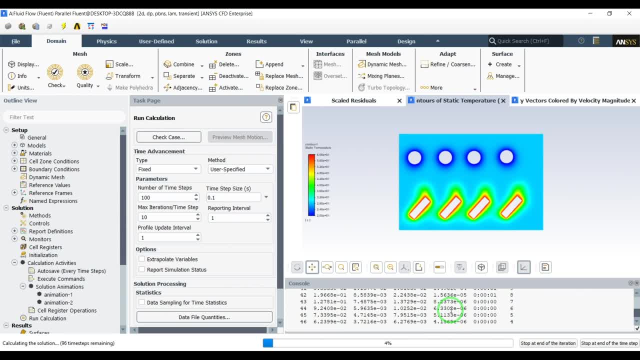 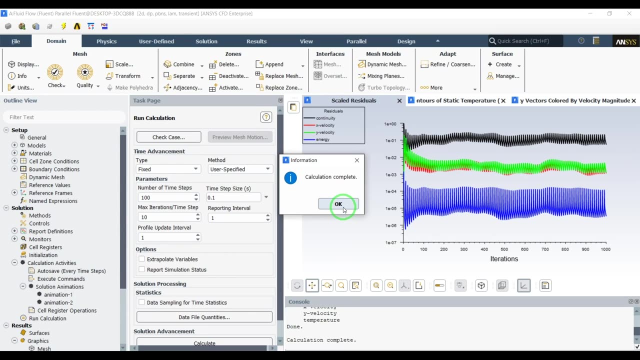 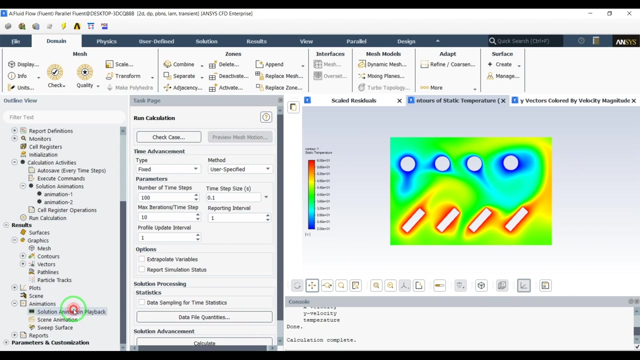 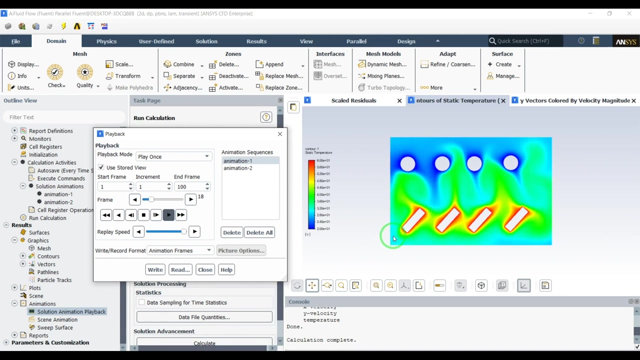 every time set, so it will take a while. so i will pause the video and come back when the simulations are finished. now our calculations are finished, so let's click ok and we'll see if the Eddy effect is right. gonna, so we are everybody now one minute forcast, um slowly. uh, i'll comment on the uh on here. 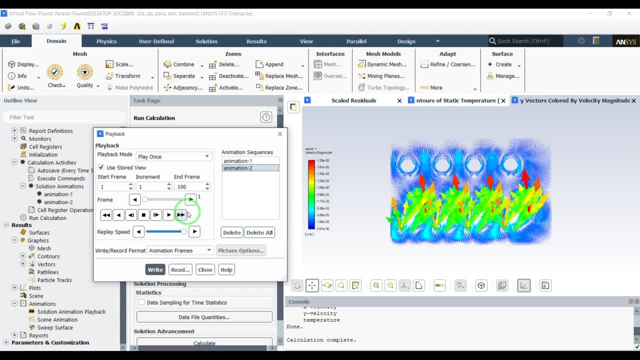 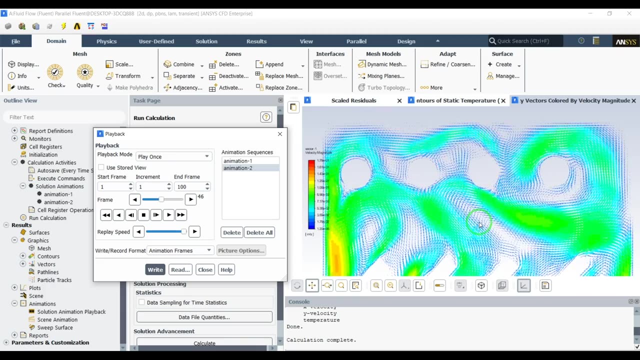 so, example, using part of an animation, you can go down to the animations and solution animations using and through that I'm called here. so let's see the velocity vectors, so you can, let's you can see some circulations here and it's very nicely showing the 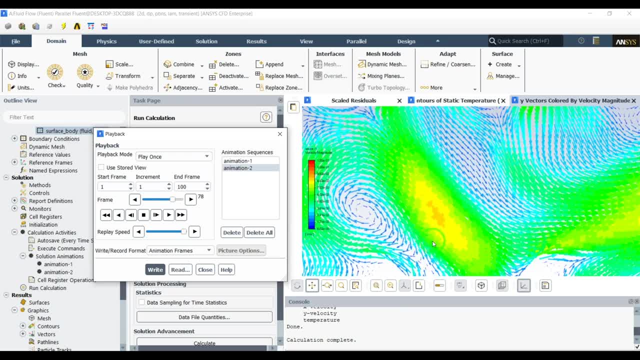 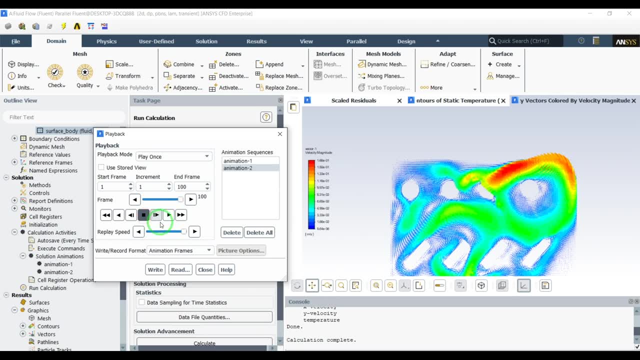 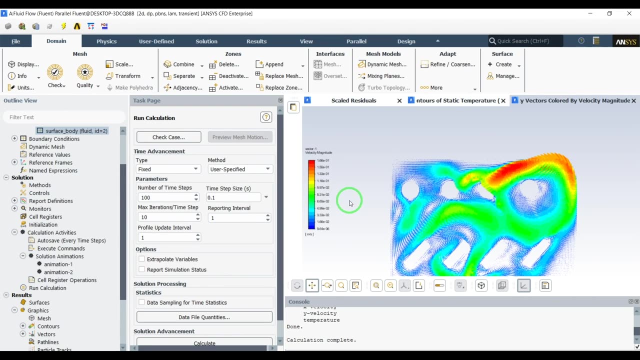 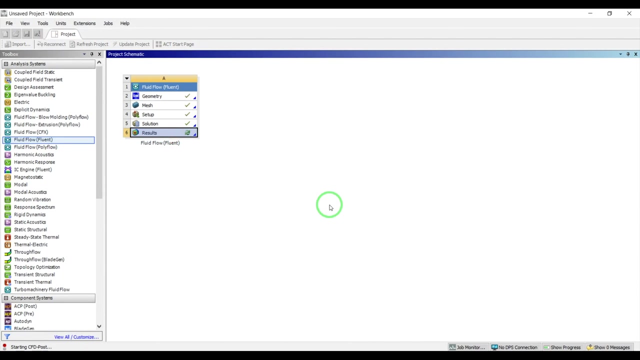 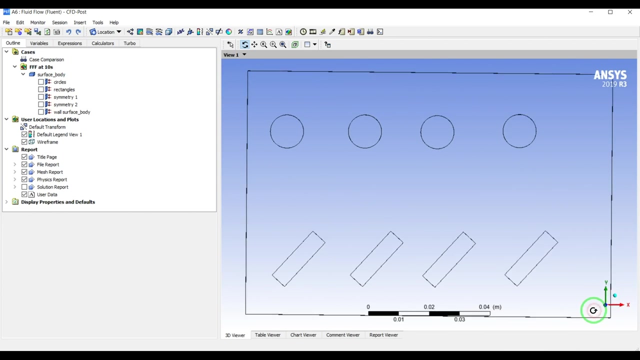 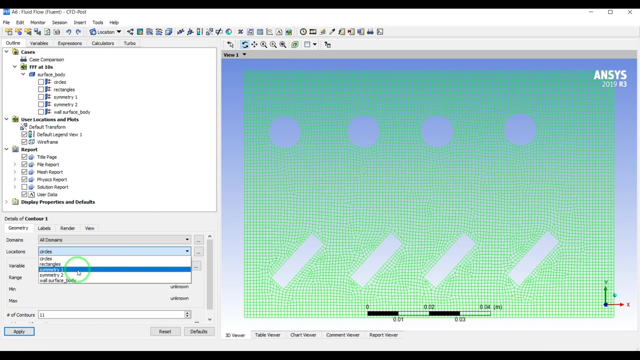 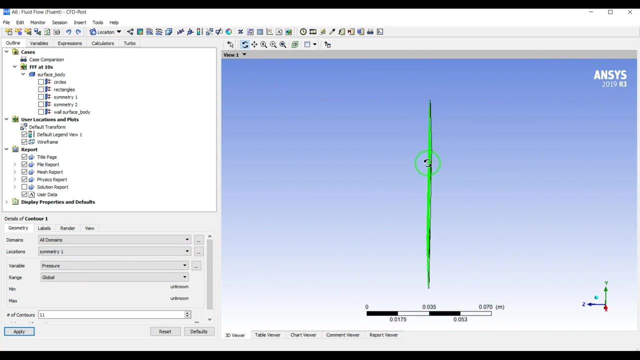 sorry about that. velocity vectors, and let's stop here. let's close the fluent and I will show you how to create the solution animations using the CFT post. we have the CFT post open. let's create a counter, so location will be in a to do. you will have a symmetry plane, because it's kinda in sub 2d, it's. 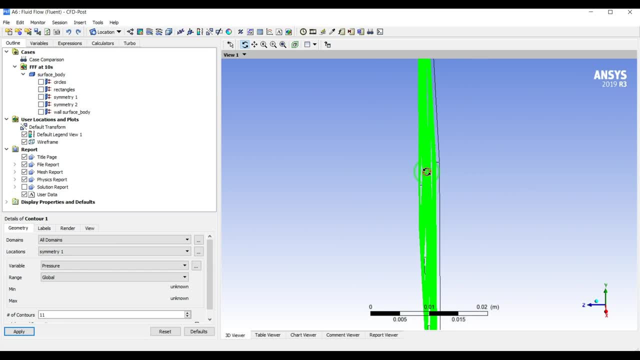 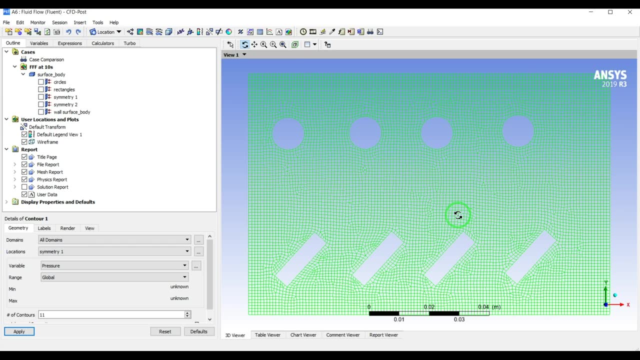 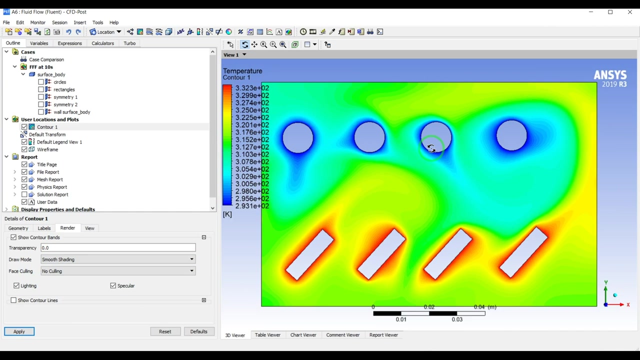 defining our geometry as the very thin 3d in the CFT post. so it doesn't matter which symmetry are using, so just select one of them. select temperature- let's have 50. let's have 50 counters and let's not have the counter lines. so looks pretty. 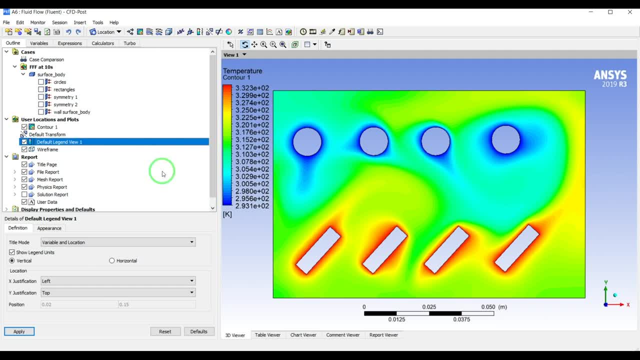 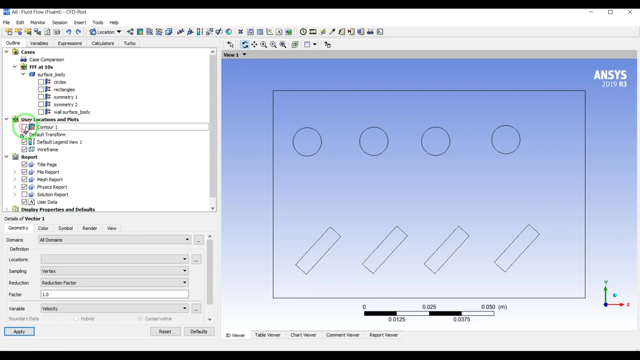 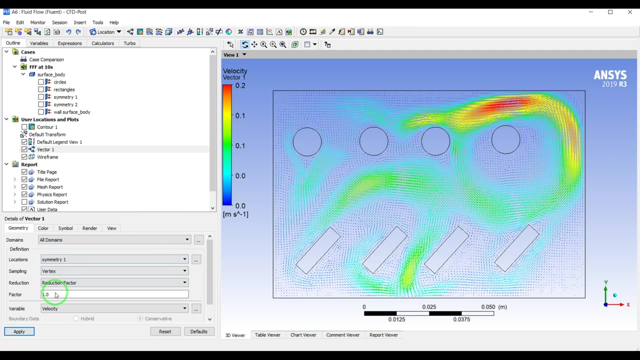 and smooth. so let's change these label views to fixed number precision one. enough so. and also we can have the vectors. let's hide this counter, so the location will be again symmetry and lost the vectors. okay, that looks nice, and now we can have a video for. 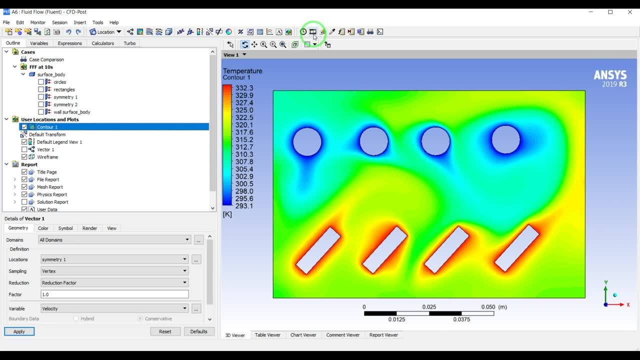 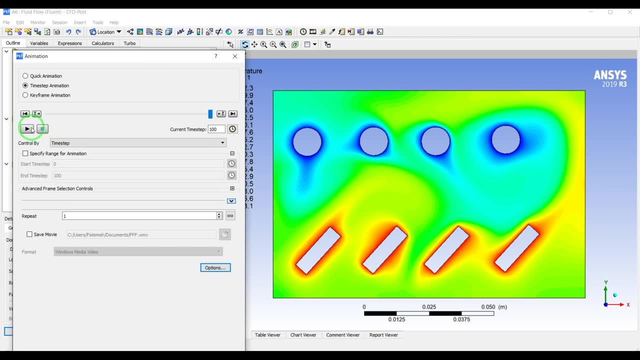 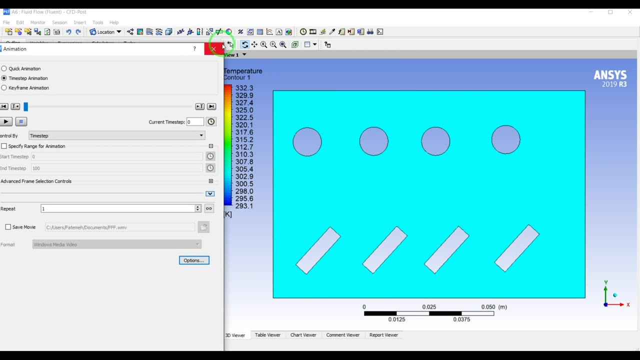 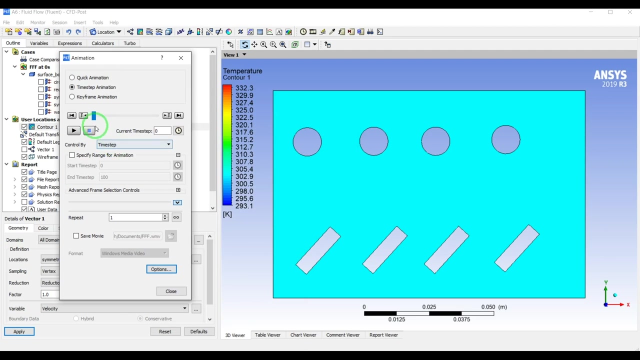 example, let's click on this video and time step animation so we can go to the beginning of our simulations. let's make this window a little bit smaller, okay so, and play this animation. so, to save this video, let's go to the beginning. go to the options here in the 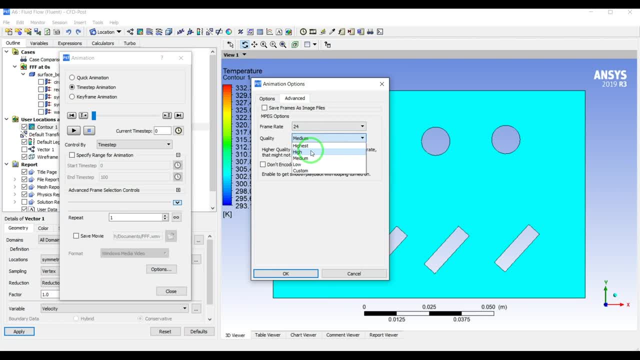 advanced. you can select it. quality: let's do the high, and this is the size of this video. you can do the edge them like HD video 7, 720 pixels or full HD 180, or we can do 4k. custom screen size: let's do the see. you can select white background. save the movie. 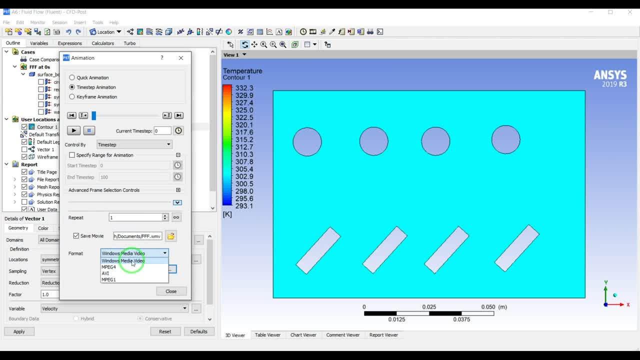 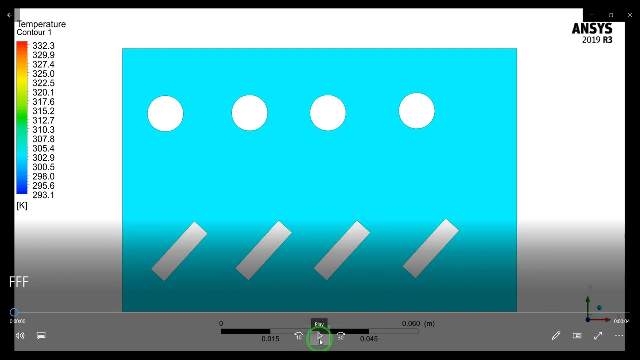 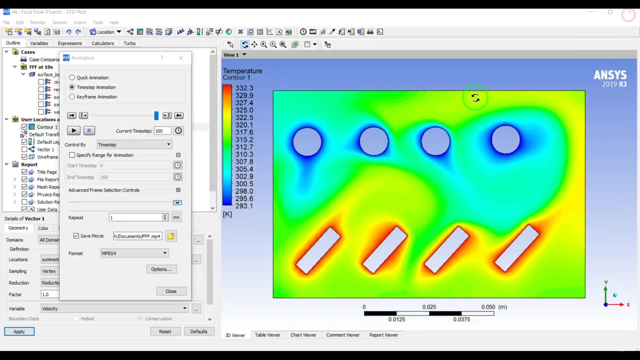 and I will do the mp4 version and when you press play to start generating the movie for you. so again, I will pause the video and play the movie when it's finished. now they are 縮읕. when your rendering is finished, you can see our. now we do have the animation. 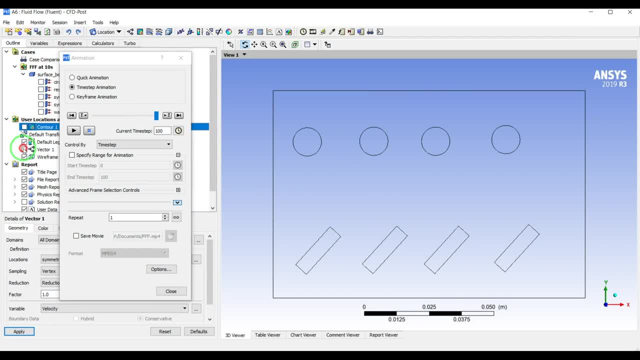 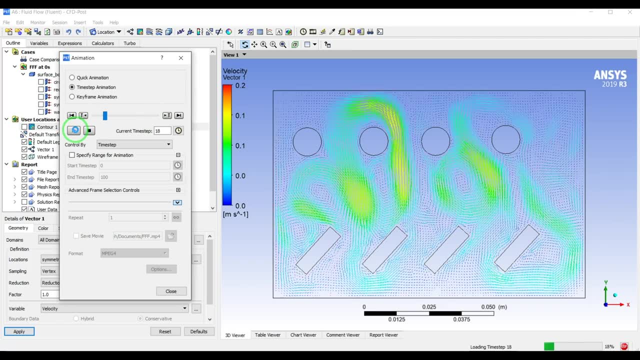 we have created. so we can like, go ahead and, for example, hide this counter and show this vectors, and we can create a video for the velocity vectors. yeah, and you can 되지 into a certain kind of animation here, whatever you want, I can also switch it to and so on, trying to say, go ahead and hide this contour and we can do all on the other vectors and we can um create a video for the velocity vectors. you can create a video. so for the vectors, we can. let's stop the video for this video. so, for example, we can copy some and put this: I third video, a ser in this should work out, and then you can forget the desyn and u ca. 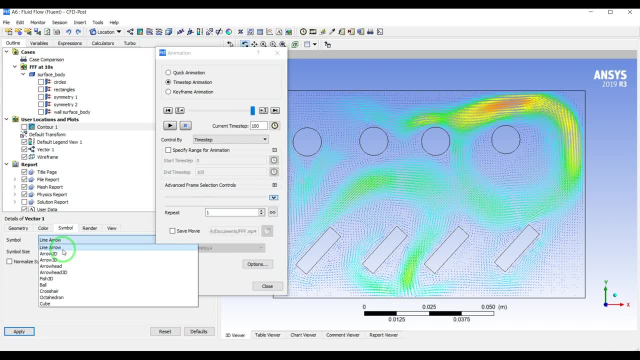 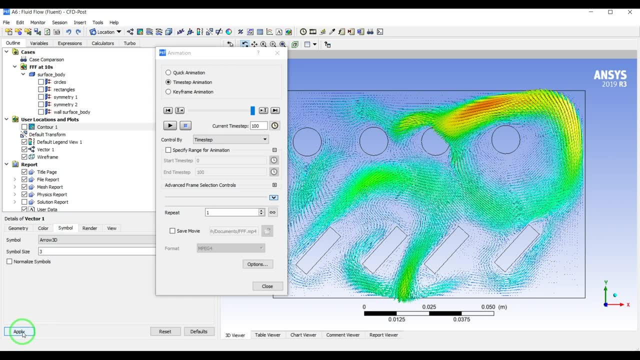 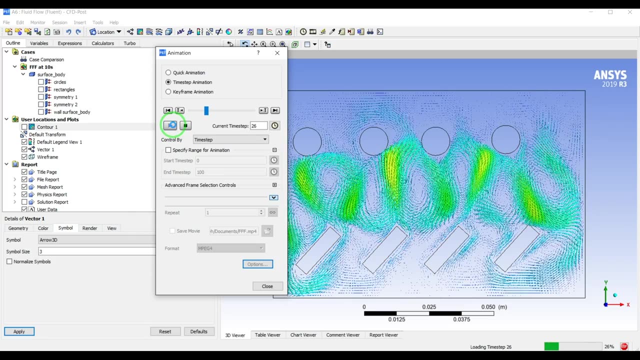 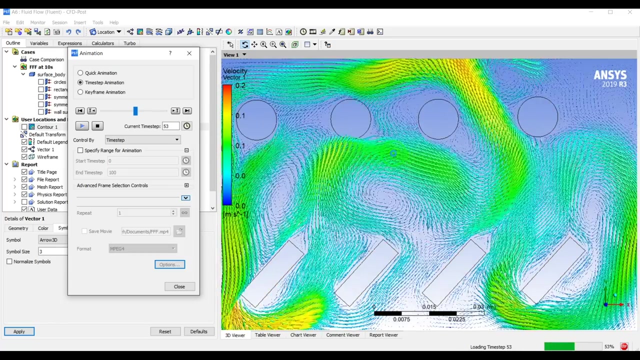 here so you can change the symbols to 3d arrow and symbol sizes to the 3 so you can see the videos. so when you use a 3d arrow it will be more intense graphically, but you can see that it's showing very nice how the vectors are. 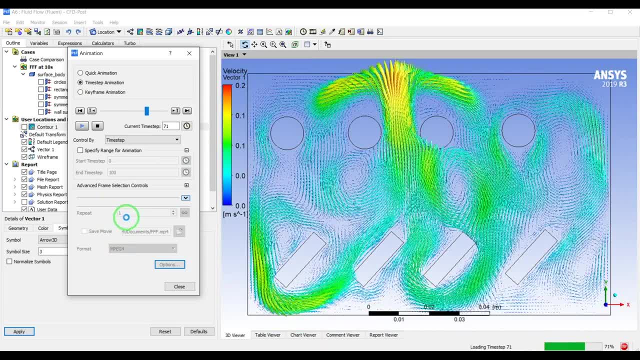 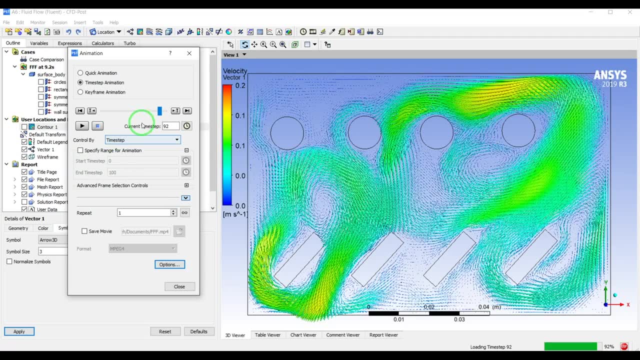 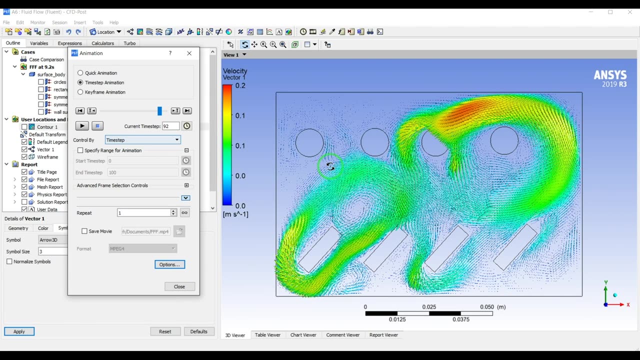 changing. you can use the same way to save this video and export an animation, and also you can create different type of post processing based on your needs. and that's all for today. thank you so much for watching this video and if you like our videos, please, please, like this video and subscribe to our channel. 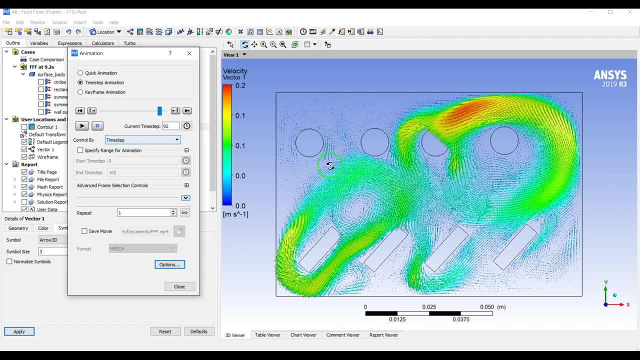 thank you and see you soon. 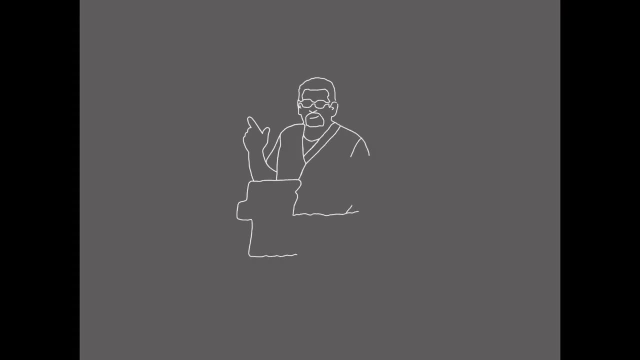 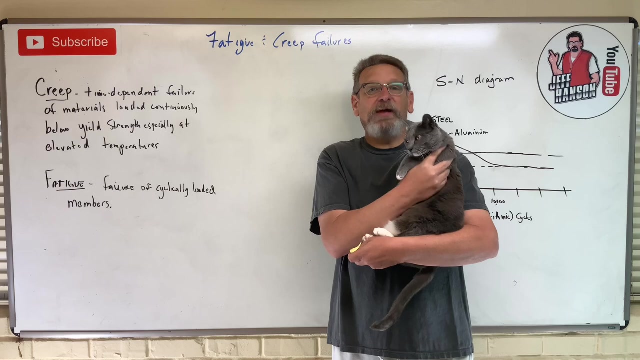 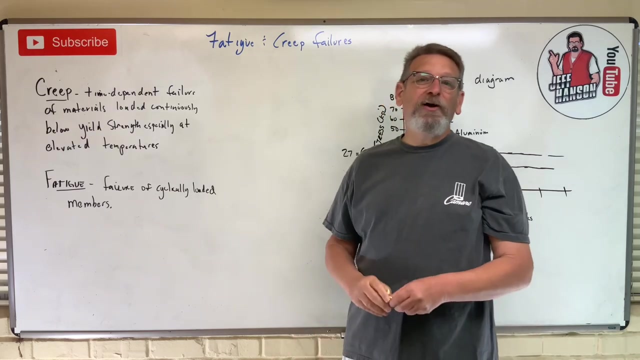 Hey my friends, Welcome back. Me and Sweetie are here to talk to you today about creep and fatigue failures. You want to talk about it? Nope, She just wants to go on. Okay, So let's talk about creep and fatigue. Typically, you're not going to get any questions over this. 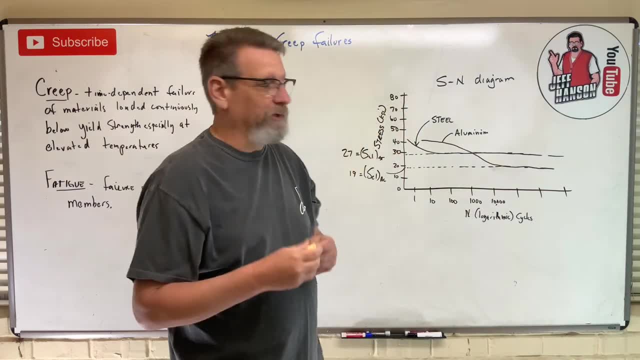 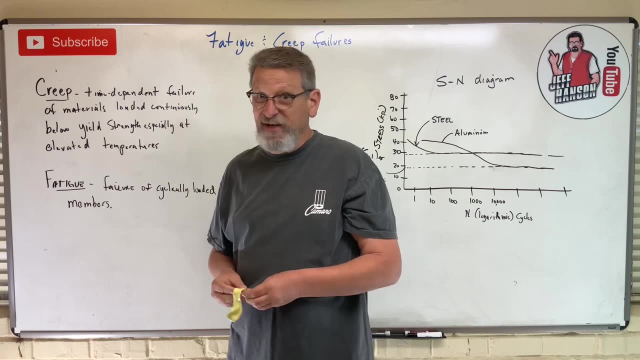 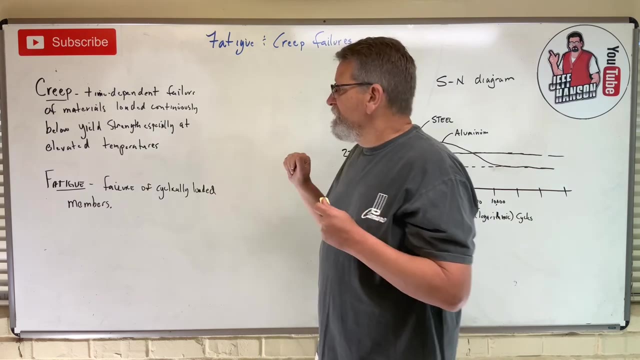 This is going to be something that you just need to understand conceptually, So I want to talk to you about it. okay, These are two kind of failure modes that we see in material science that don't come from just a pulling or applied force. okay, So what is creep? Creep is a time-dependent